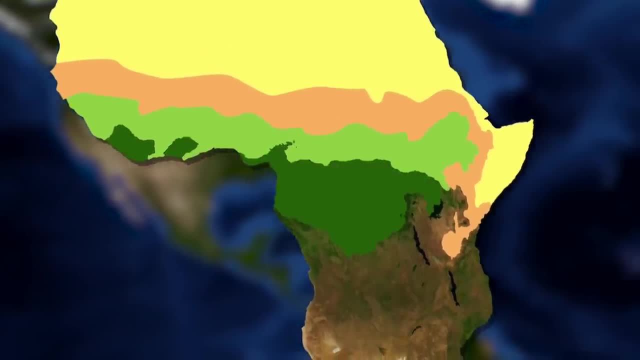 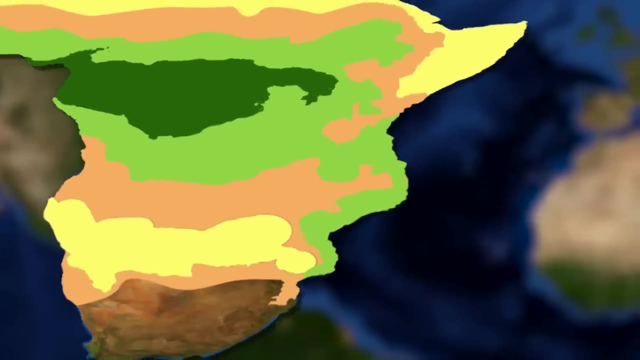 comes grasslands which eventually finally become forest. At this point we have crossed over the equator and we begin to find more grassland, then more semi-desert, Another full desert and then finally back to the Mediterranean climate we found at the 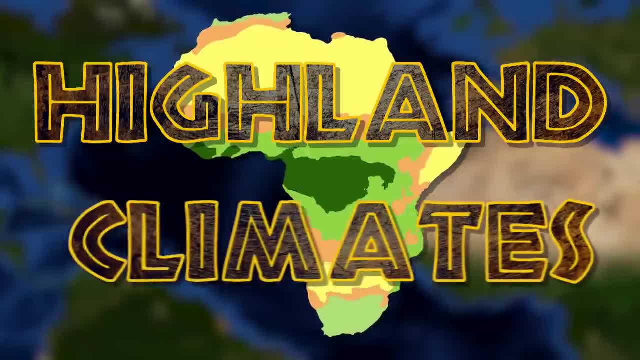 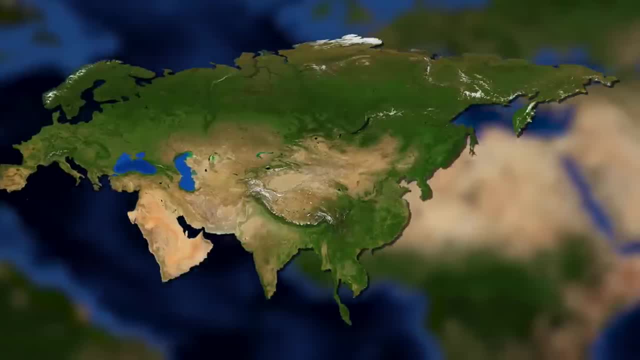 northern tip of the continent. Then add in features like highland climates, where there's highland arid, semi-arid, semi-humid and humid, and you have a very fractured landscape. Compare this to Eurasia, which has a polar climate, a temperate climate, a small Mediterranean. 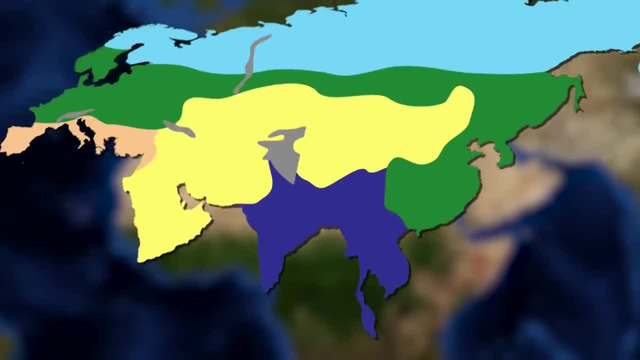 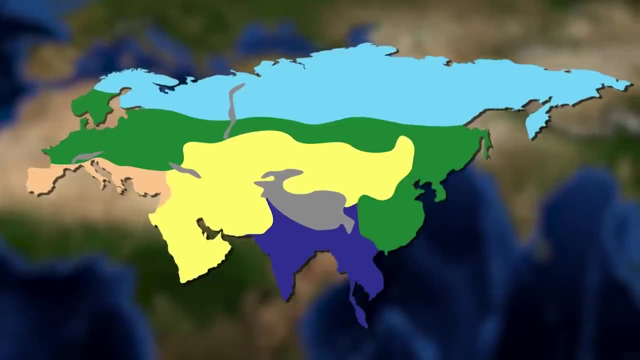 climate: a desert and a tropical zone. There are some alpine areas as well, most notably the Himalayas, but even still you can see these massive areas of single climates form, And each one roughly corresponds to the size of the entire continent. 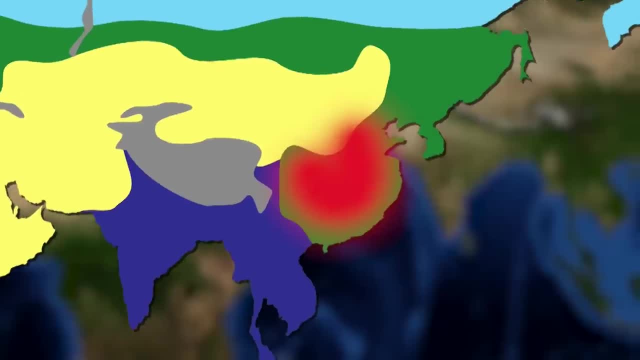 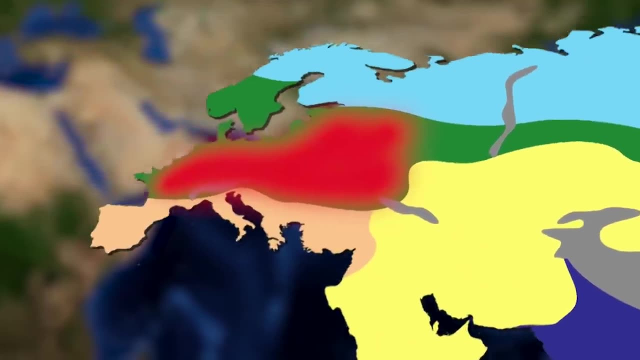 So if you want to know more about Eurasia, check out the description below. So the eastern temperate zone became China, while the tropical zone to the south became India, The desert became the Muslim Empire and the western temperate region became the. 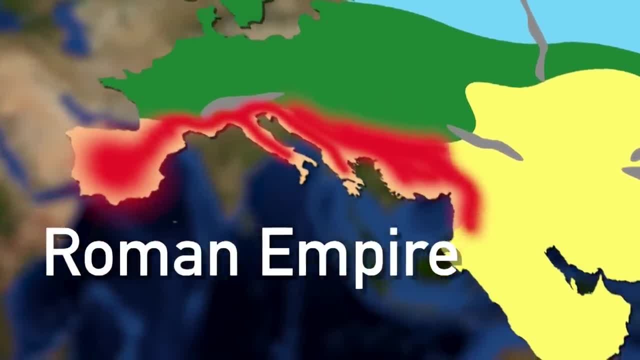 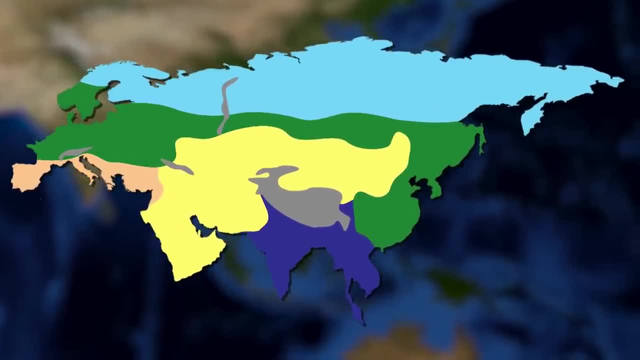 powers of Europe. The Mediterranean also roughly corresponds with the heart of the Roman Empire. What all of this shows is that large areas of the same climate allow civilizations to unite, grow and thrive. This happens because people who live in a single climate survive. 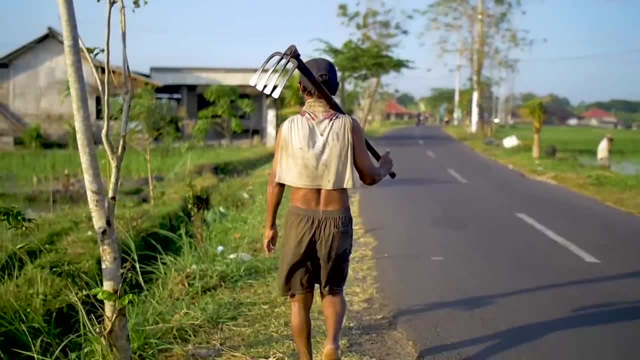 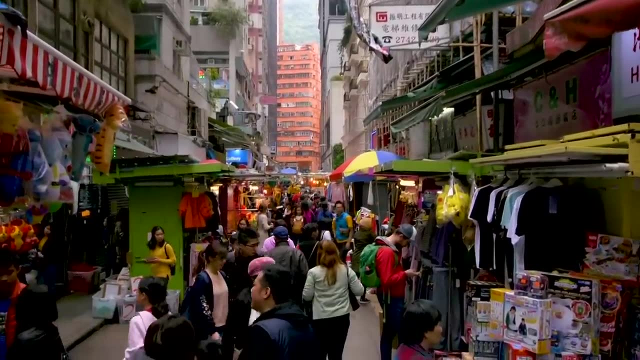 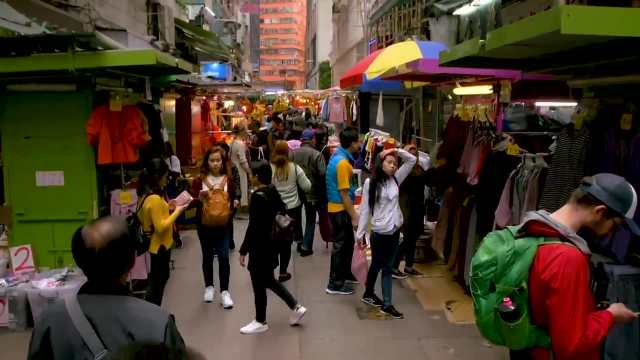 by farming and hunting the same foods, experience the same hardships and therefore live in very similar ways. This allows them to interact with each other, forming a common language and systems of interaction like trade and defense from outsiders. They develop the same lifestyle and end up sharing a common culture without even trying. 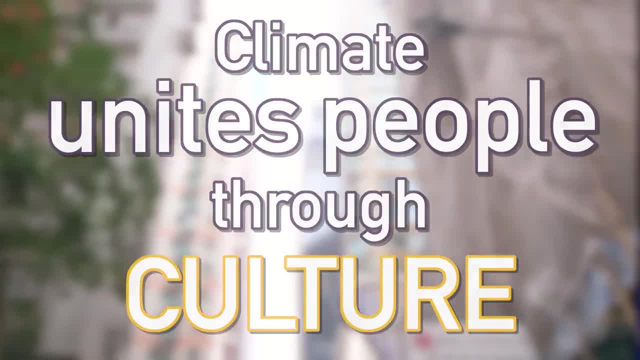 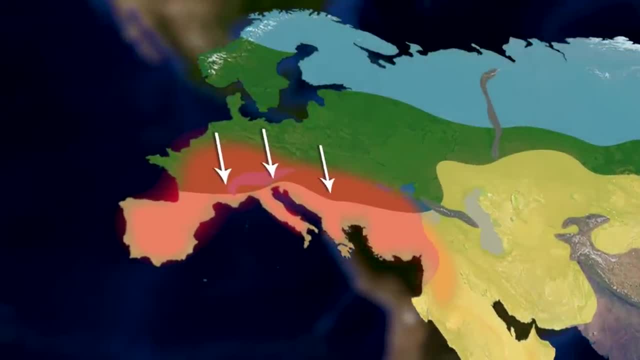 In short, climate unites people through culture. It's interesting to think that the reason the Roman Empire failed was because of invaders from the north who lived in a different climate zone and therefore held different values and cultures than the Romans, who tried to conquer them. 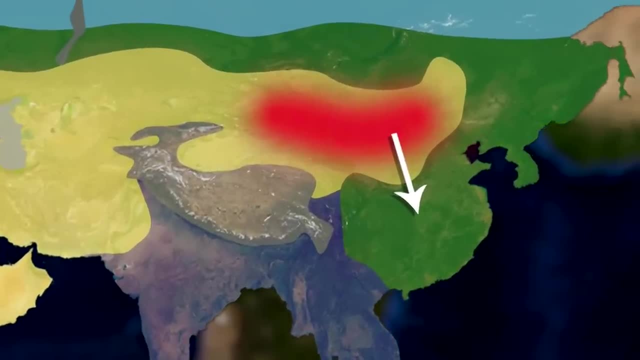 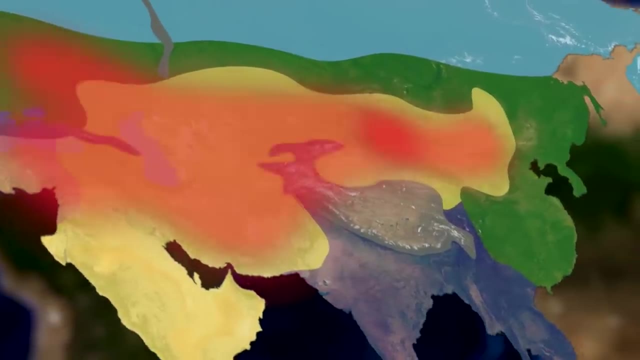 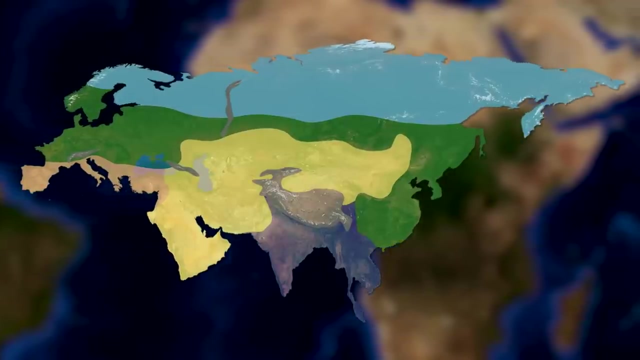 who invaded China never permanently ruled, also being from a different climate zone, while they did have great success conquering westward where the climates were roughly the same. It seems these places were destined to remain independent, in large part due to their unifying geography, which made them resilient to outside forces. But in Africa you didn't really. 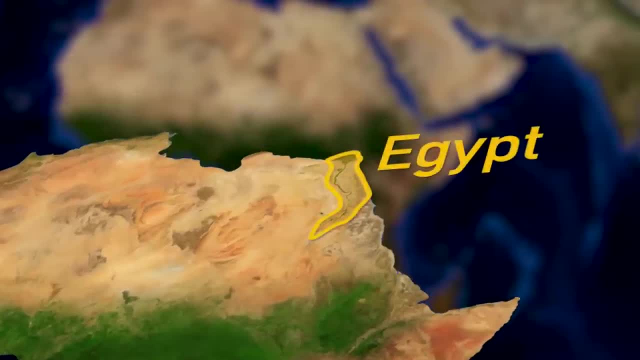 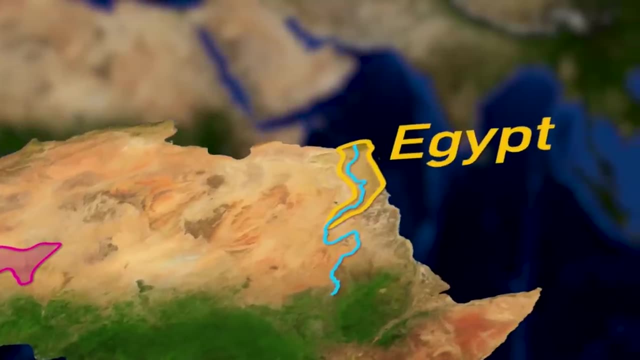 get this. Of course, some empires emerged. States like Egypt and Mali experienced times of great power and prosperity, but Egypt was locked to the Nile and was never capable of expanding much beyond the river valley, and Mali straddled the narrow Sahel region between the Sahara and the 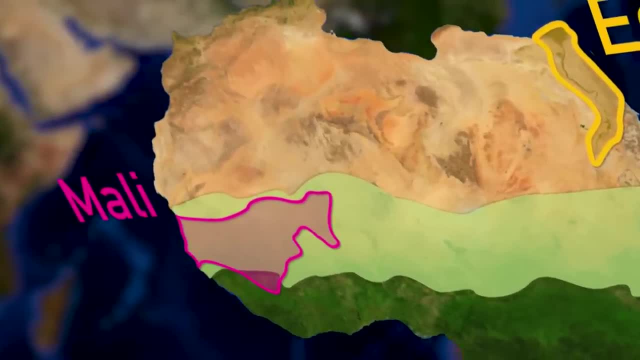 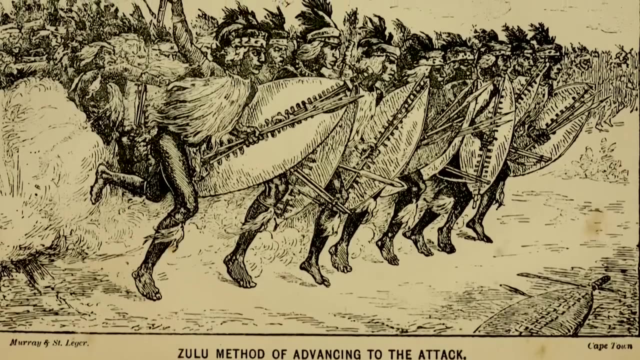 tropics, which was much larger centuries ago, but still limited. Beyond their lands, they found people with vastly different lifestyles and cultures who would resist assimilation by different cultures, and they became trapped by their own climate, unable to expand and develop further. 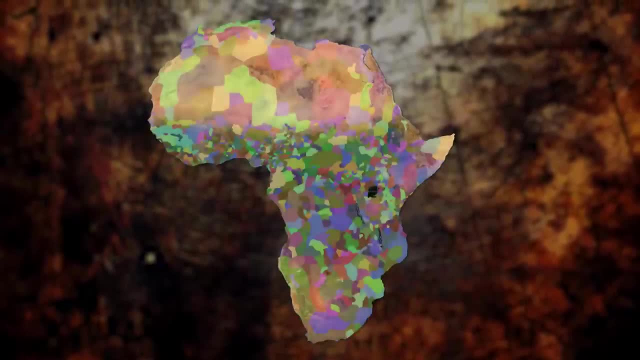 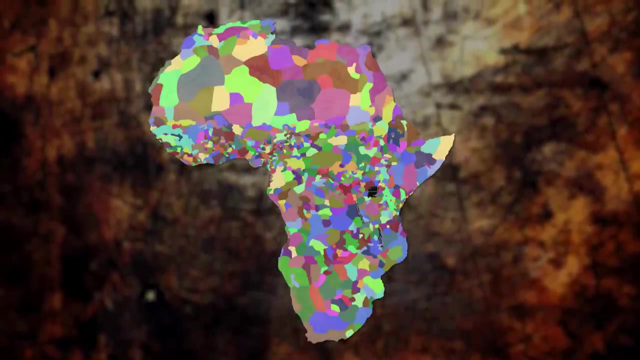 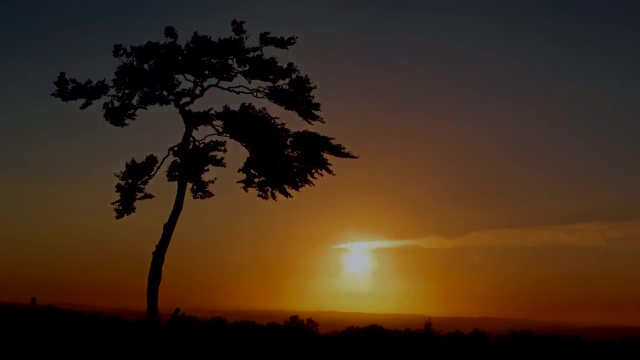 A map of individual African culture groups would look something like this, with thousands, thousands of tribes and clans, each one distinct and therefore opposed to joining forces to resist all outside powers. This also caused small tribes to never develop much trade beyond their neighbors, and therefore new ideas and technologies could not easily diffuse through. 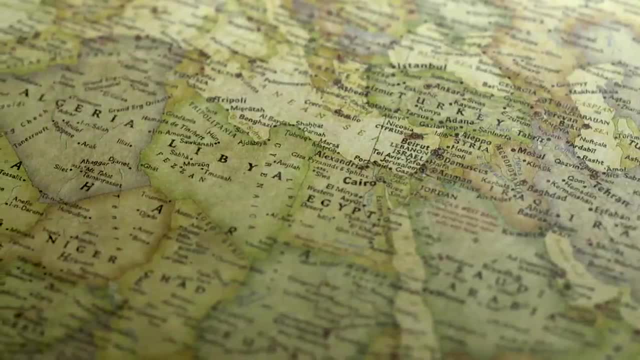 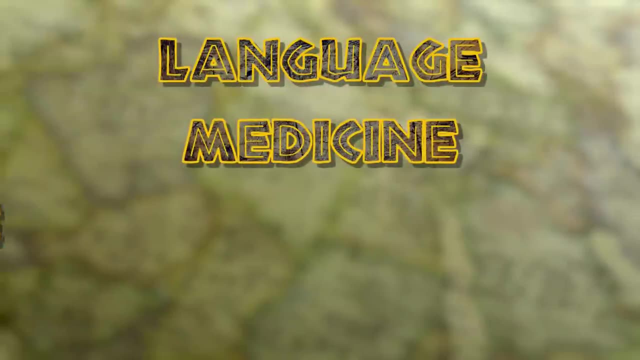 Africa the same way they had between Europe, the Middle East and Asia. That's not to say, Africa didn't have innovations of its own, And actually many of mankind's earliest advancements in language, medicine, architecture and mathematics came from Africa, But without large-scale. 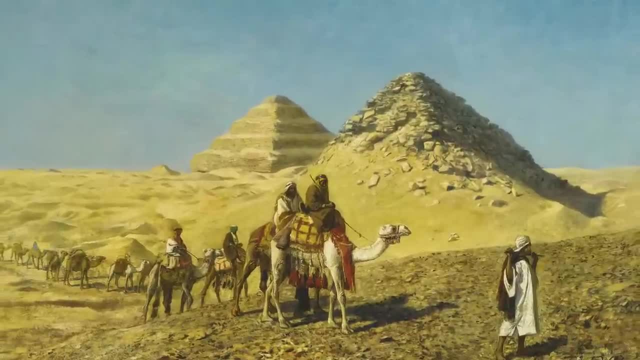 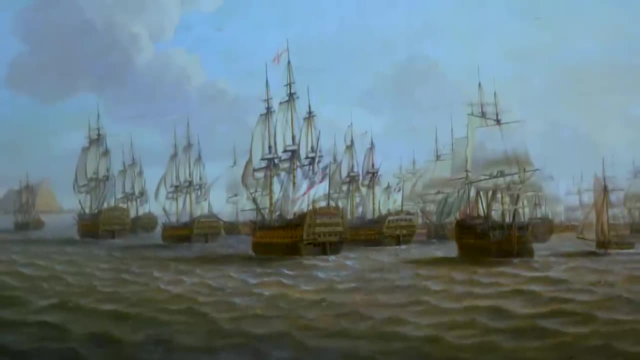 exchange, Africa would not have been able to survive. As the world changed throughout the continent and with other civilizations, these advancements were impeded and the numerous tribes of Africa fell behind technologically. By the 16th century, Africans were confronted by people who had benefited from a unifying geography and trade. 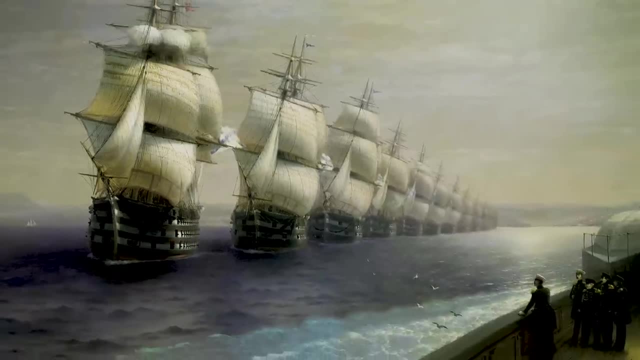 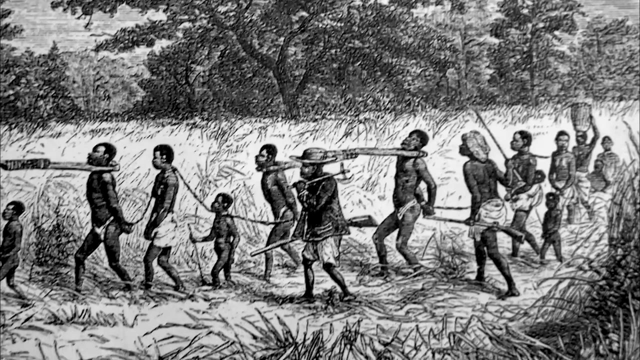 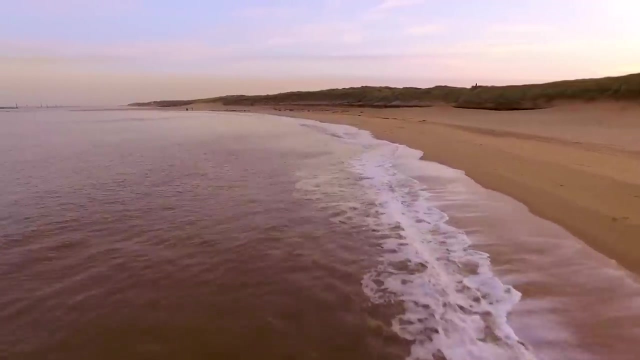 with distant lands. They wielded guns, sailed on massive ships and completely overpowered local populations. Africans fell victim to harsh colonial rule, while foreign powers competed to take advantage of the land that had doomed its own inhabitants. Because Europe was smaller and relatively poor in resources, Europeans were forced to seek outside their own lands. 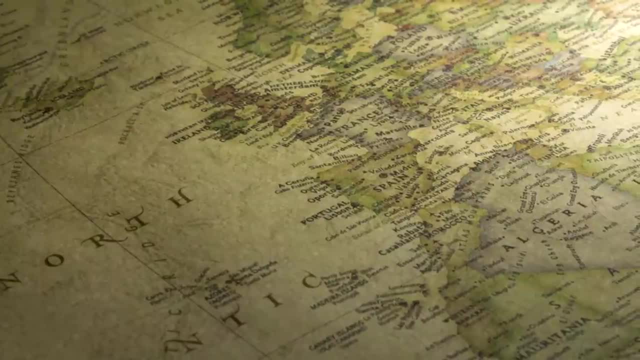 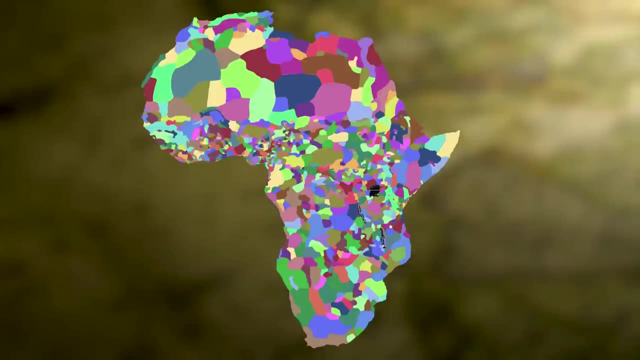 to advance their civilizations. So geography both caused the Africans to lag behind and also encouraged Europeans to push out beyond their own lands. Then the colonizers grouped the people into arbitrary borders, So desert tribes could be paired with a Sahel and a. 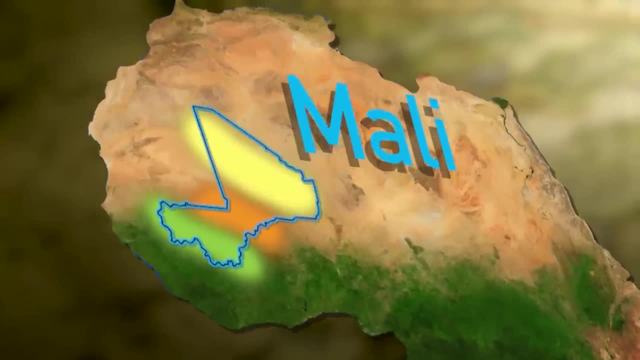 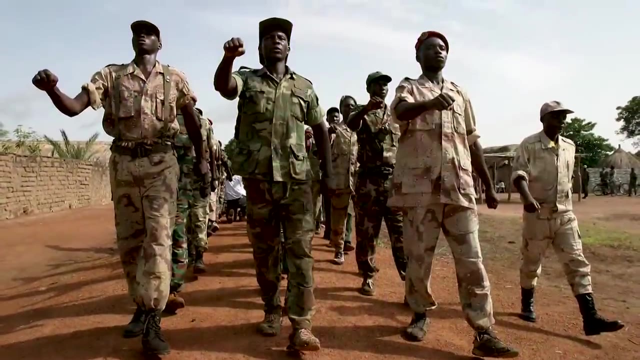 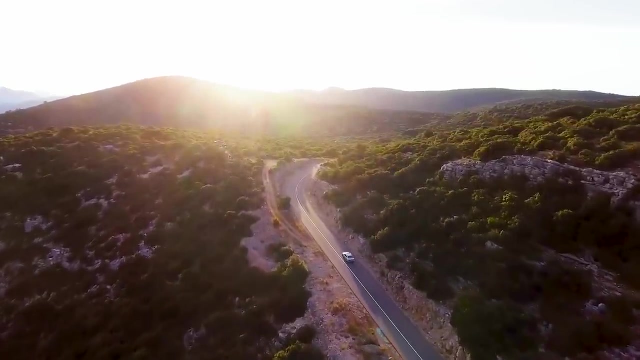 forest tribe and told they were one, like in the modern country of Mali. This, of course, led to internal issues within basically every African nation. Revolution and civil war has followed in nearly every state since colonization And you can see the countries that have had the most success today are the ones that lucked. 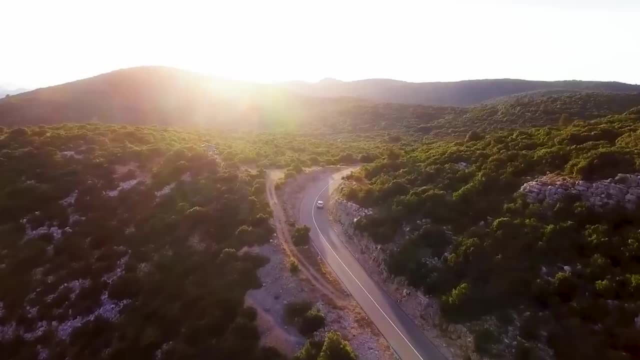 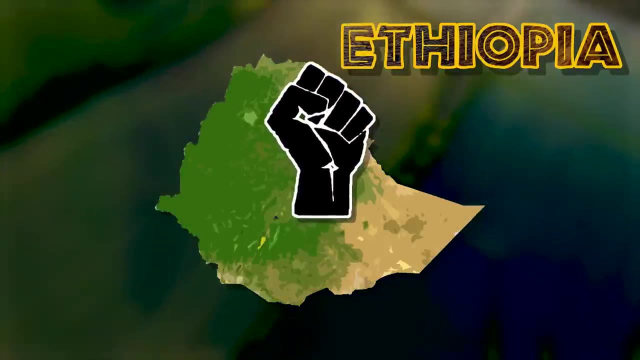 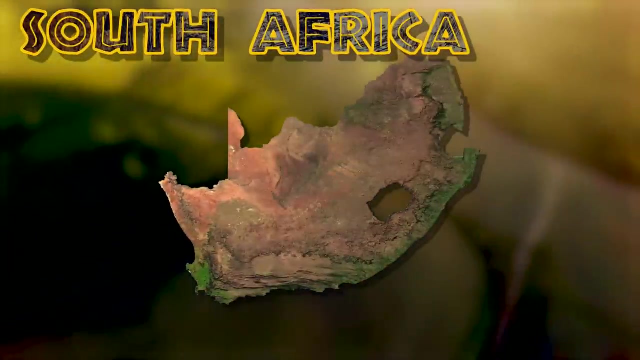 out and ended up with borders that coincided with the natural climate zones. These included nations like Ethiopia, which, for the most part, is humid and mountainous and managed to maintain independence throughout colonization, Egypt, which is all desert surrounding a single river with a long history of unity, and South Africa, which is mostly semi-arid Mediterranean.